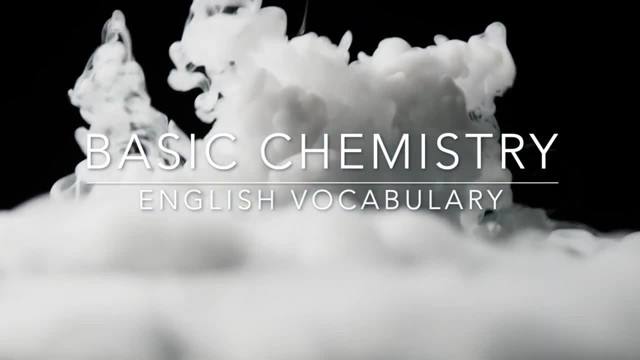 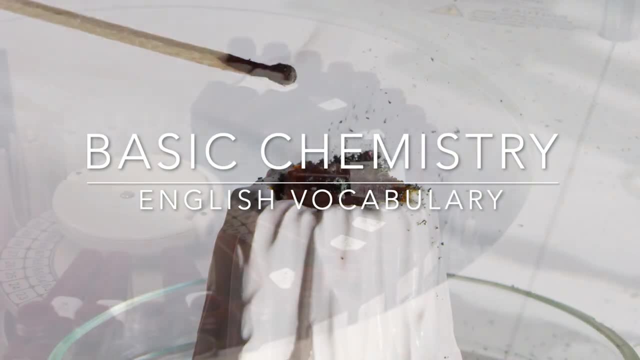 Hello everyone and welcome back to Learning English Pro. Today we're diving into the fascinating world of basic chemistry. Chemistry is all around us, from the air we breathe to the water we drink. So let's get started and explore some essential chemistry vocabulary. Make sure. 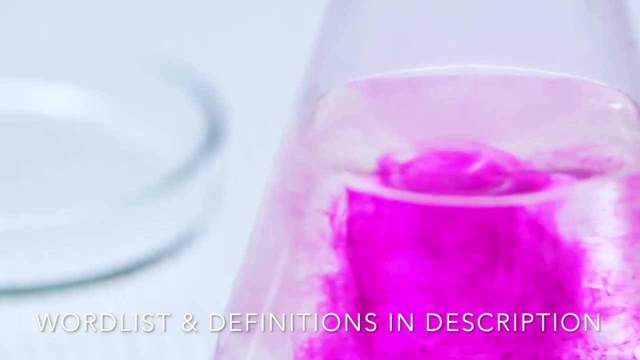 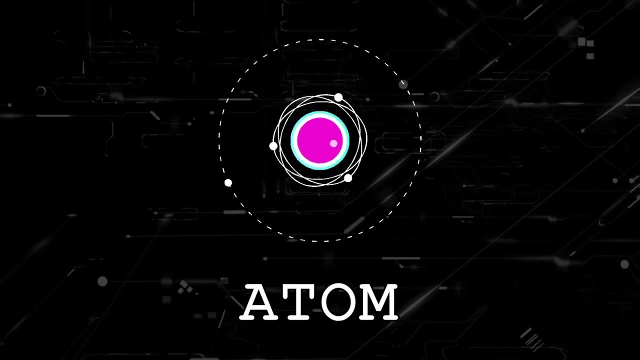 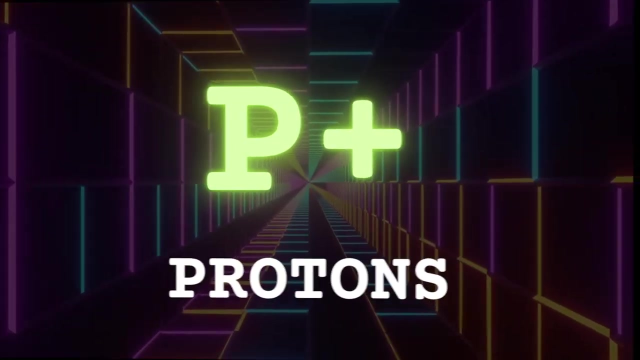 to check out the complete word list and definitions in the description of the video. So if you're ready, let's jump right in, and our first word is atom. An atom is the smallest unit of matter. It's made up of a nucleus which contains protons and neutrons, and they're 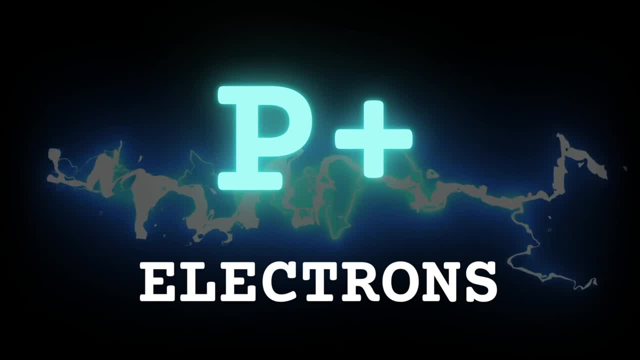 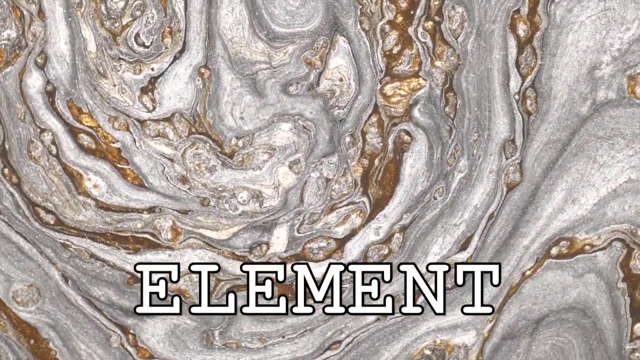 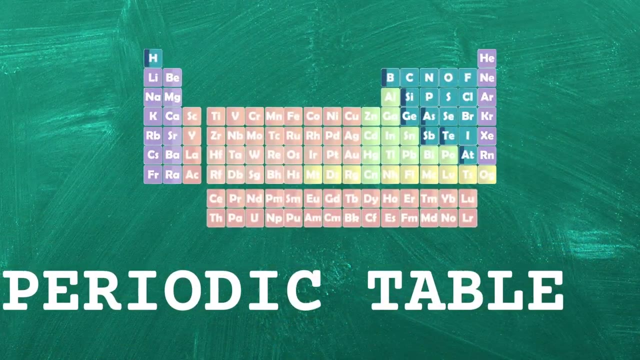 surrounded by electrons. Moving on to element, an element is a substance that consists of only one type of atom. Examples include hydrogen, oxygen and carbon. Now let's explore the periodic table. This is a periodic table of elements and it's just a periodic table. It's not the periodic. 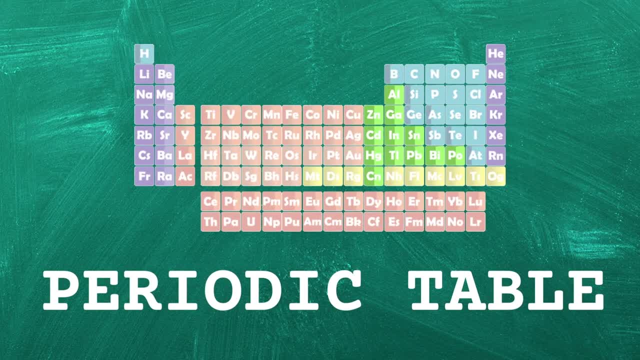 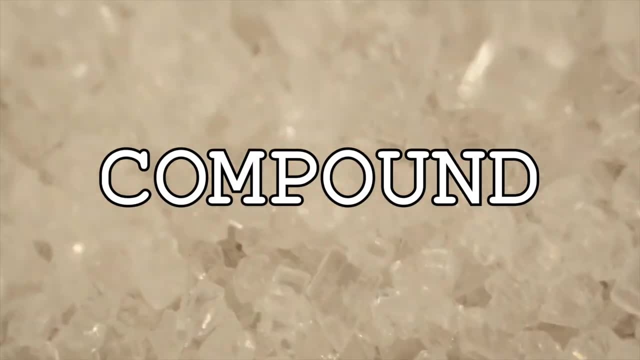 table that you see on the screen. It's a periodic table of elements. It's a periodic table that tabular arrangement of all known elements, organized by their atomic number and properties. Next we have compound. A compound is formed when two or more different elements chemically combine. 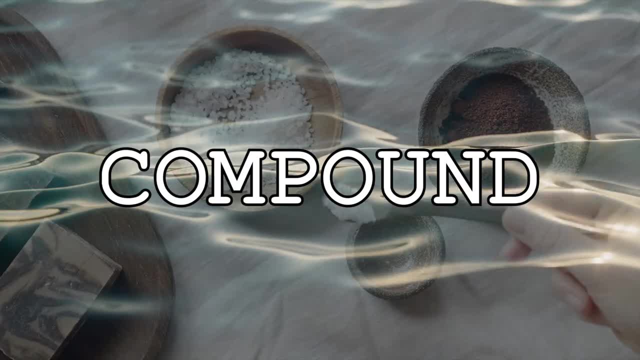 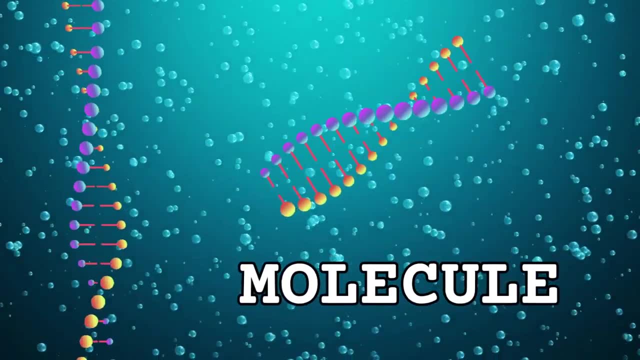 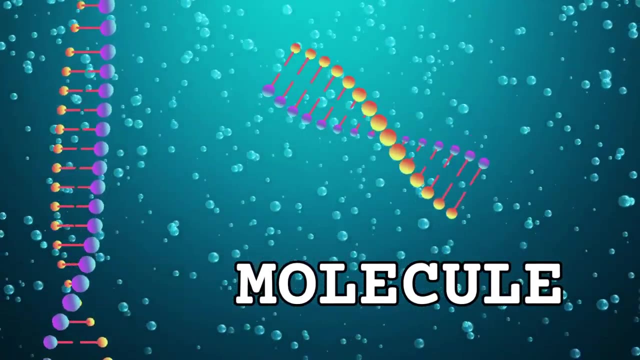 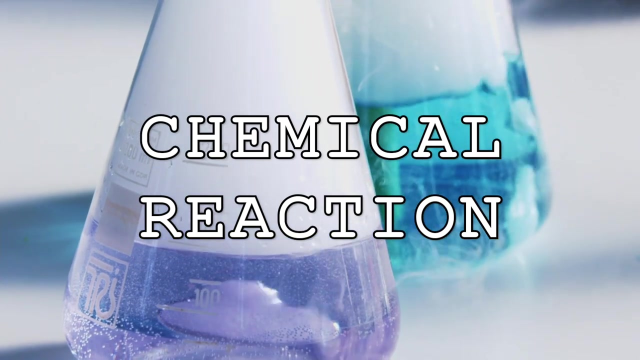 in a fixed ratio. Water, or H2O, is a well-known compound. Molecule is our next term. A molecule is a group of atoms bonded together. Oxygen gas and glucose are examples of molecules. Moving on to chemical reaction, A chemical reaction occurs when substances interact. 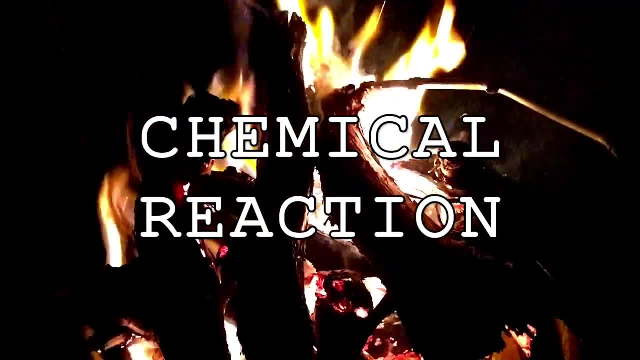 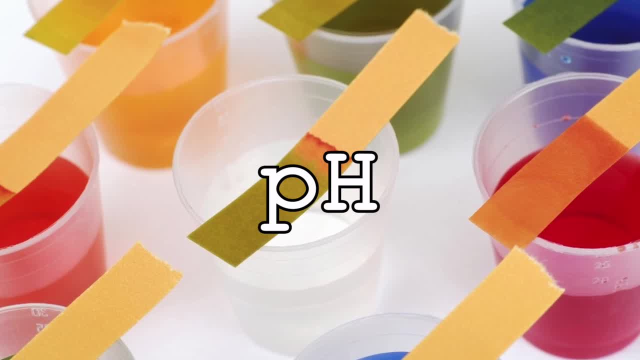 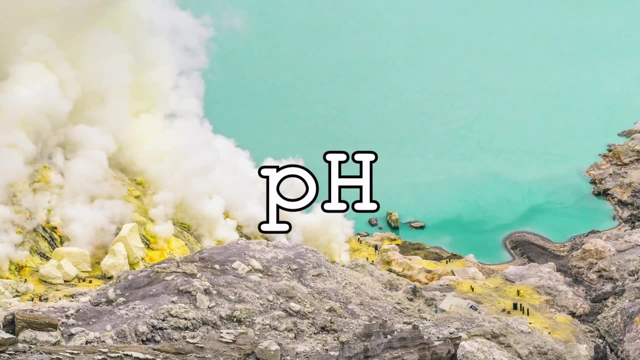 to form new substances with different properties. Think of burning wood to produce heat and ash. pH measures the acidity and alkalinity of a solution. It's a scale ranging from 0 to 14, where 7 is neutral, lower values are acidic and higher values are. 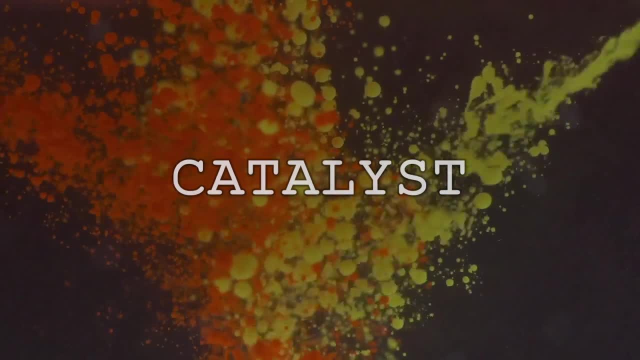 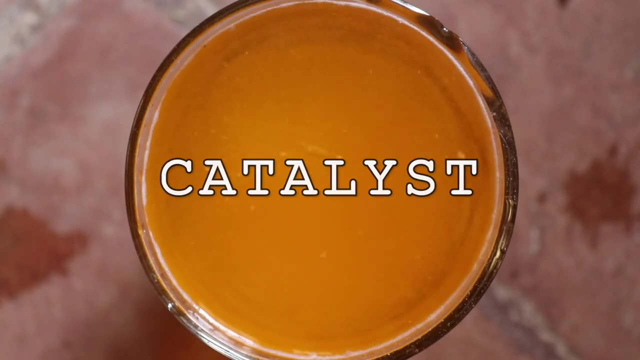 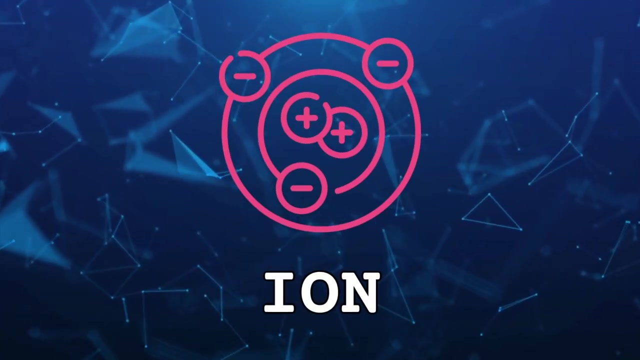 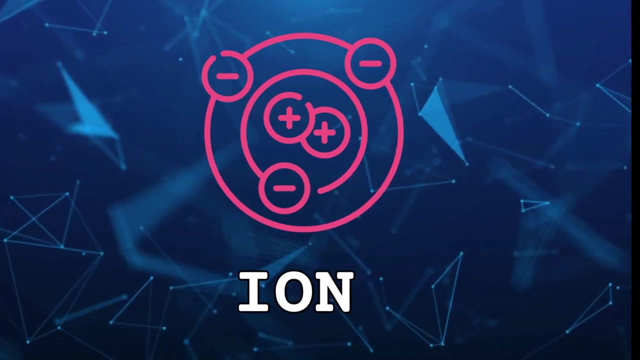 alkaline Catalyst is another good term to know. A catalyst is a substance that speeds up a chemical reaction without being consumed itself. Next up is ion. An ion is an atom or molecule that has gained or lost electrons, resulting in a net electric charge. Chemical bond refers to the